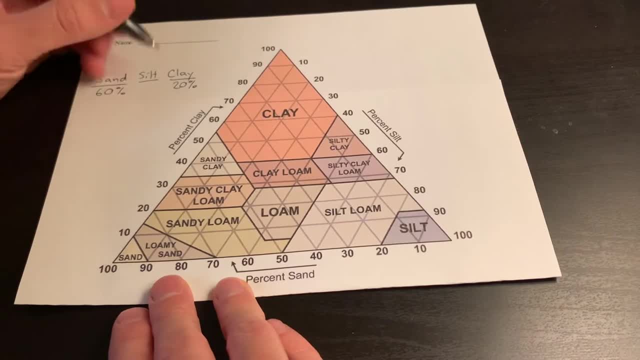 CHORESUPS, PAUSES, ONE MORE TIME. IT DOES NOT END CREATING UP AFTER ONE. CAN We have an box which is at the bottom, pushing up and standing second and second in the middle, where the core stick is most easy? what percent silt should we have? we know that it needs to add up to 100. 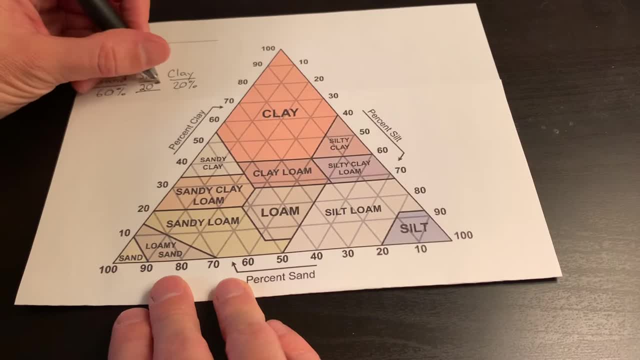 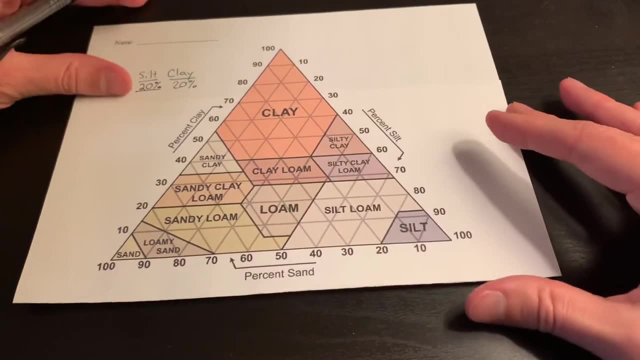 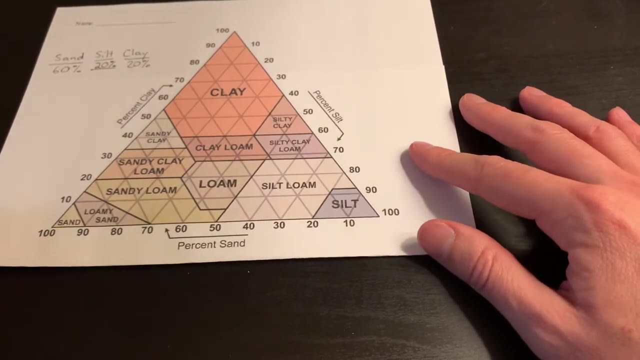 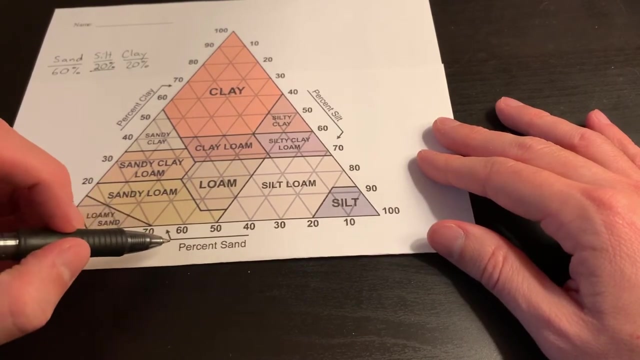 so we know we should have 20 percent silt because all three of these should add up to 100.. so if we've got 60, 20 and 20, we'll consult our soil texture triangle and for the sand, notice how it says percent sand and then see this little arrow pointing in this. 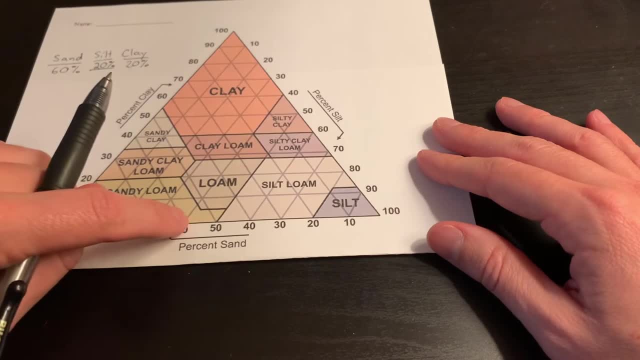 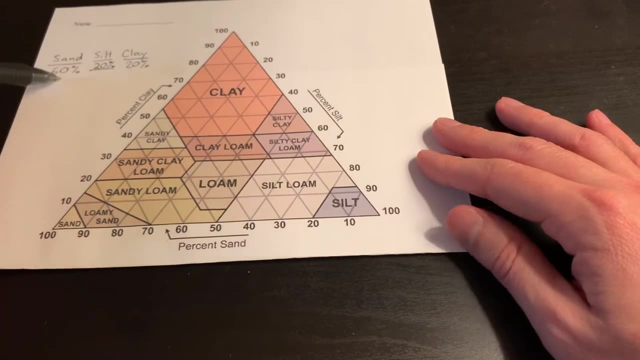 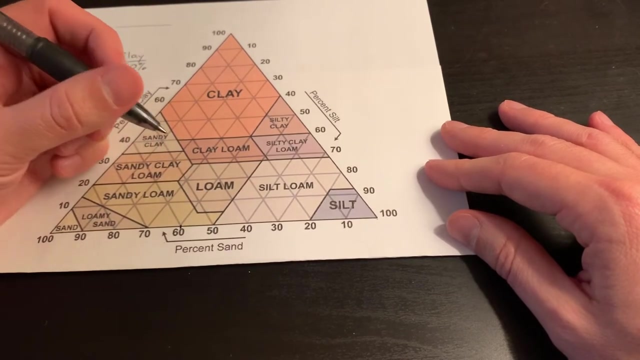 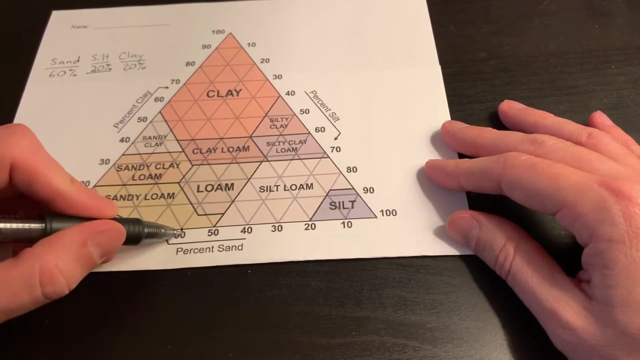 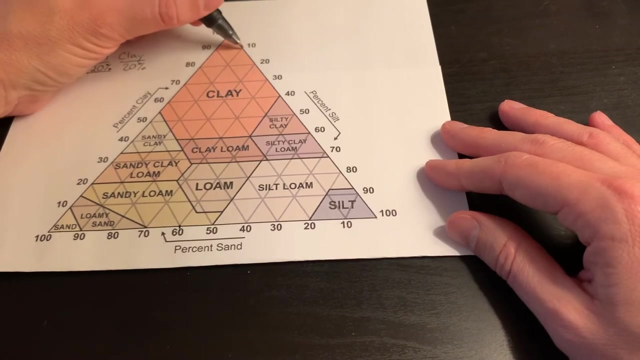 direction. that is telling you that we are going to read our lines in this direction. so we take our 60 percent sand and we find 60 percent on the triangle and we are going to read that in this direction. for sand, if we take our percent silt as 20 percent, we come up here and here is percent silt. 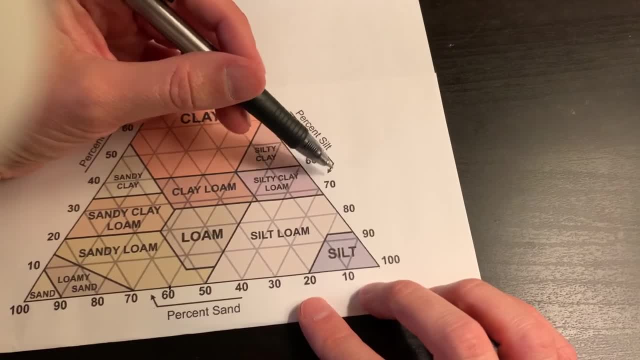 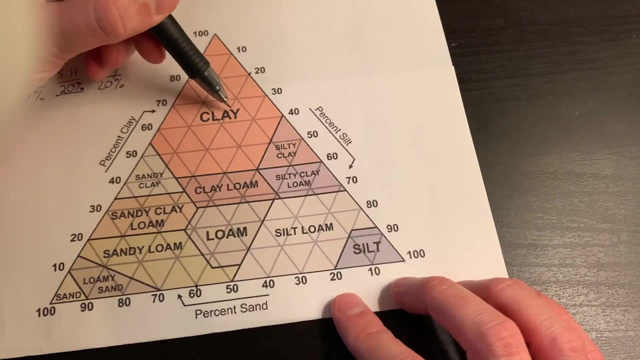 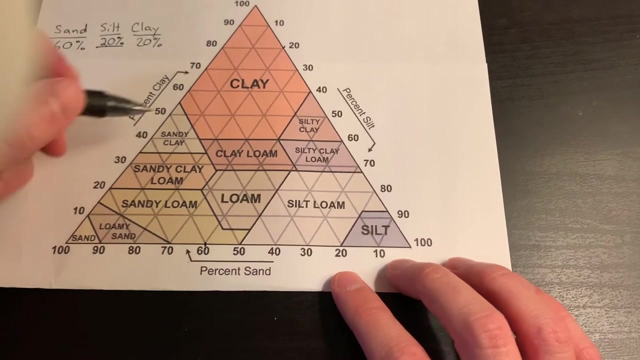 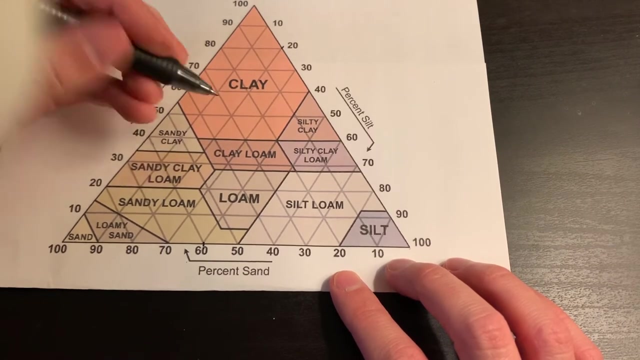 at 20.. notice, this arrow is pointing down in this direction. so that means we are going to read silt down this way. so if we take the sand at 60 and bring it up this way and bring the silt at 20 and bring it down this way, we follow the lines until they intersect. 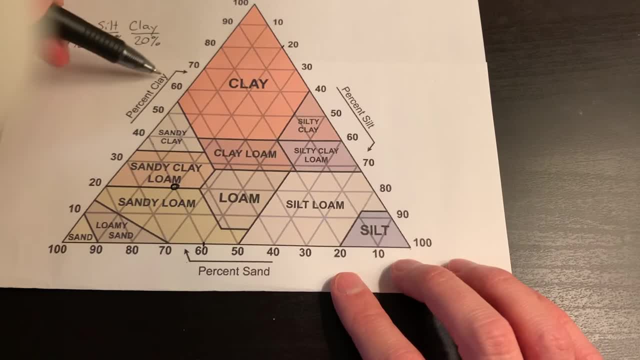 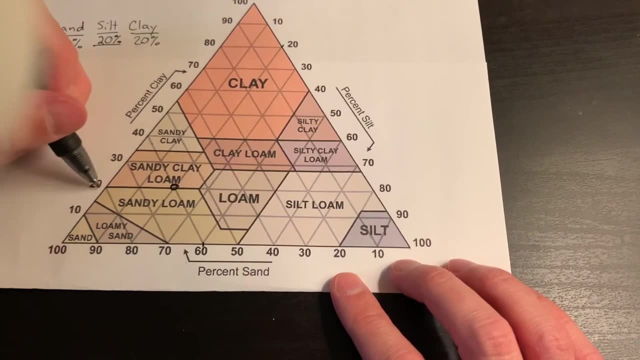 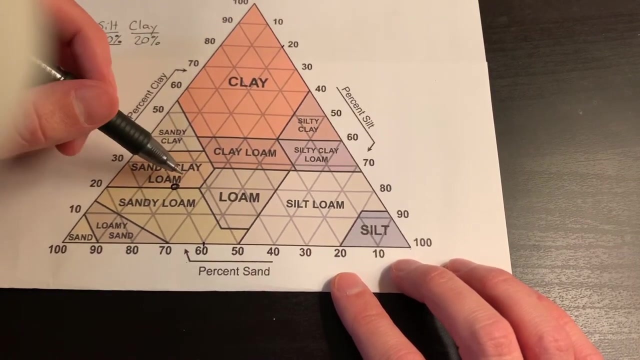 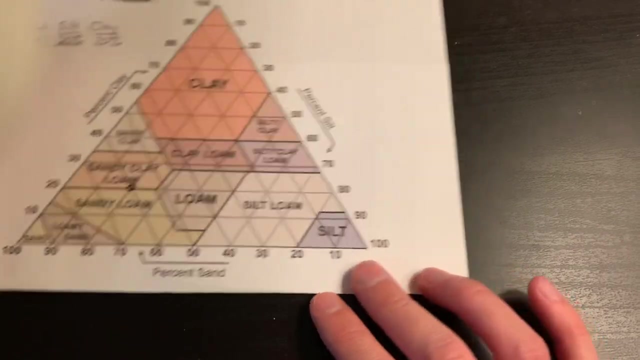 and to check that we did it right, we look at our third piece here: percent clay, see the arrow going horizontal and so we go up to clay 20 percent. so for this first example we are right on the edge of a silt. now you'll see how we are in the middle of our triangle at 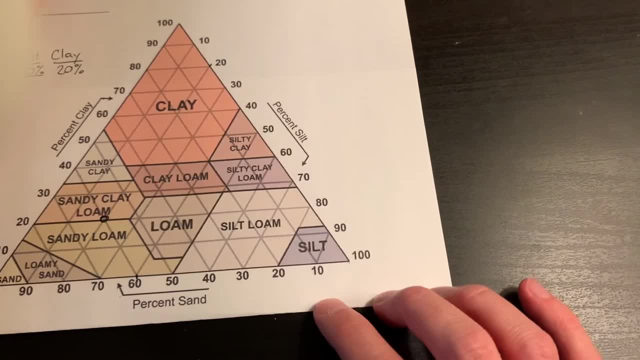 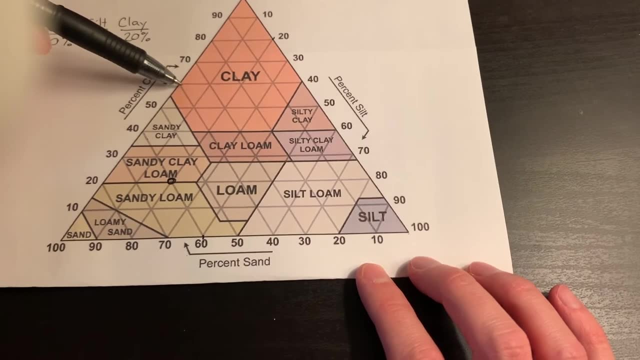 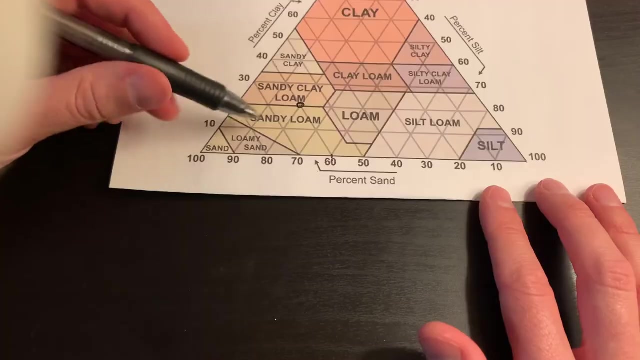 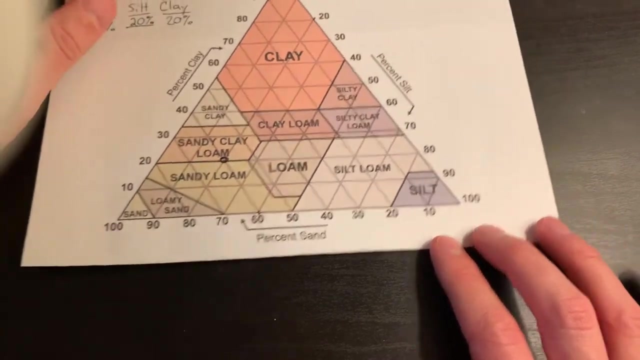 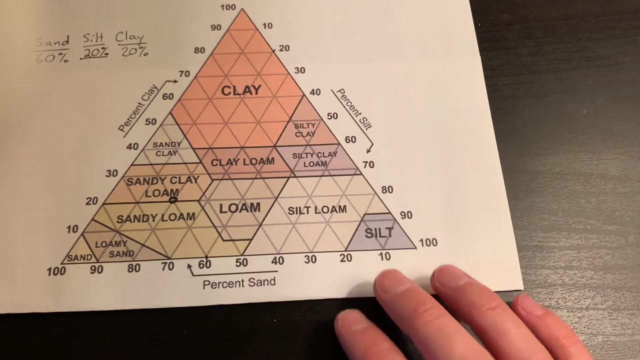 just 1.3. now we are passing on the silt of the triangle at 20.. Whereas if you have more than 90 percent sand, that is the only thing that will make you a pure sand. Let's do one more, just to practice. 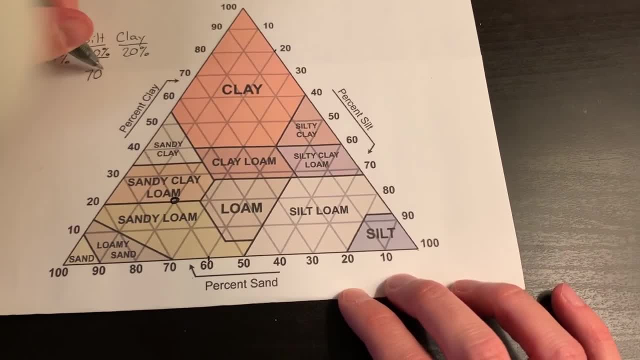 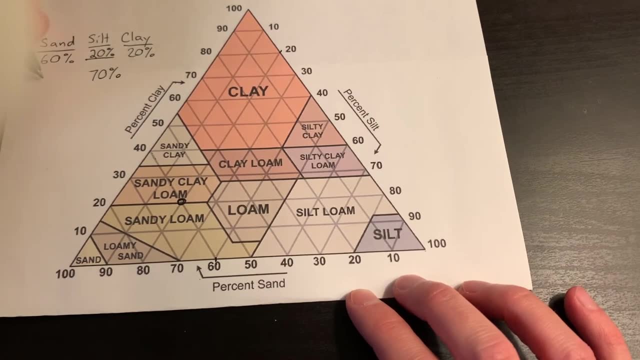 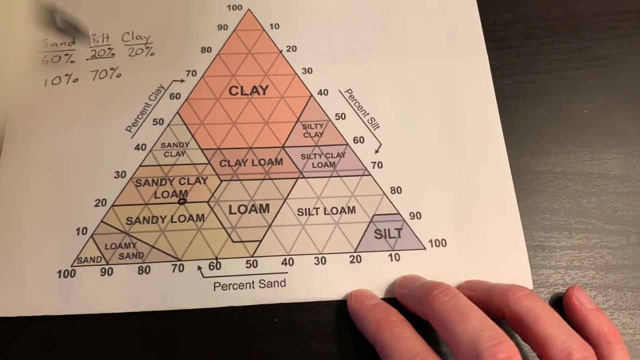 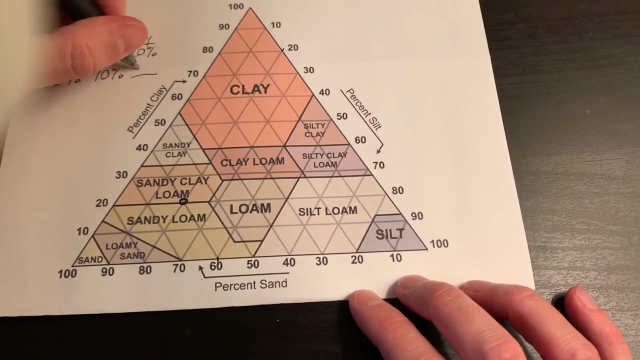 So let's say that we have 70 percent silt and that we have 10 percent sand. So if we have 10 percent sand, 70 percent silt, how much clay should we have? Again, 20 percent. So we take our sand. 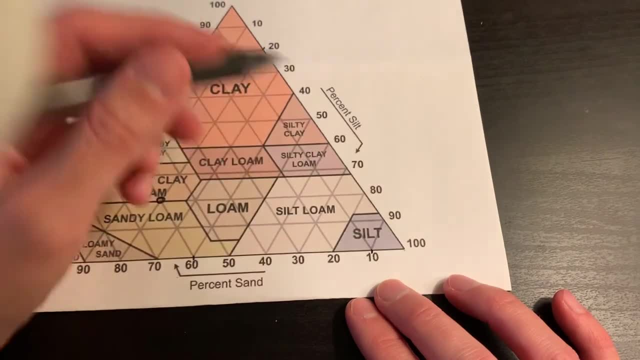 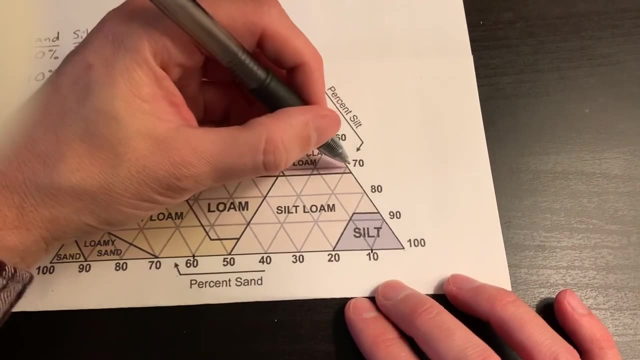 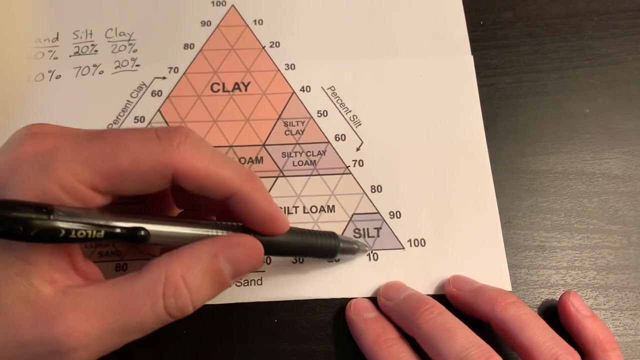 And we look at our silt And we look at our 10 percent. So we're going to be coming up on this line. We take our silt and we find 70 percent and we're going to be coming down on this line. 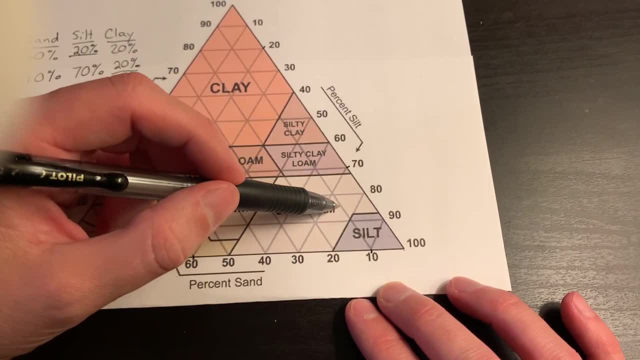 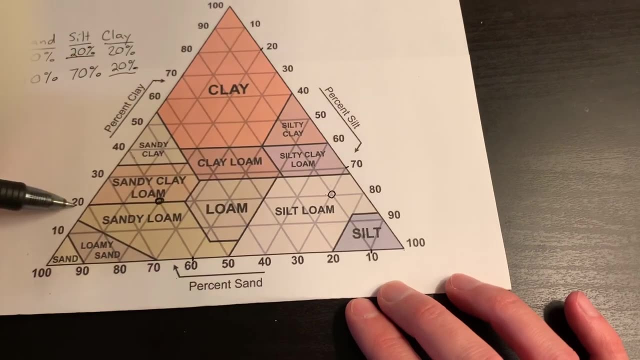 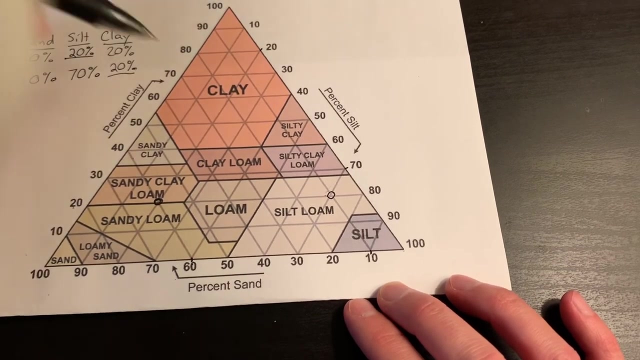 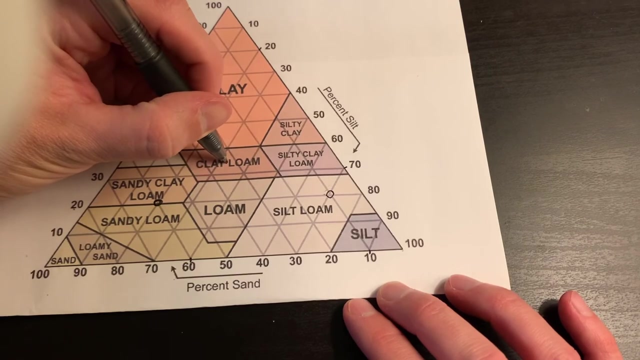 So if we have sand and silt, we double check that With our clay percentage it all adds up to 100.. So for this soil we are a silt loam. We can work in reverse if we want to know what is a clay loam. 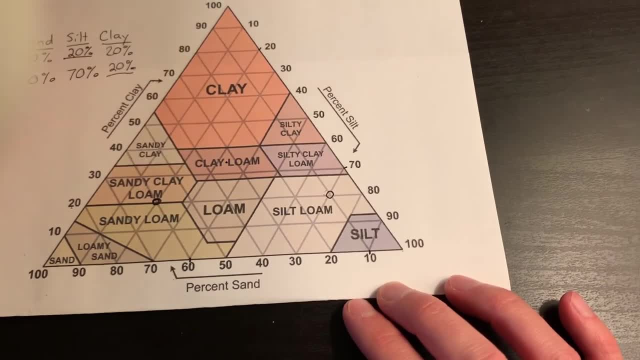 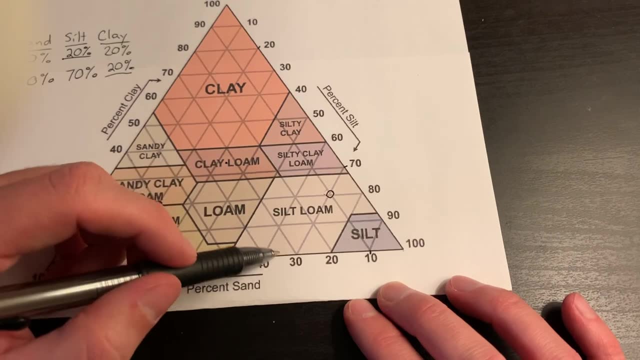 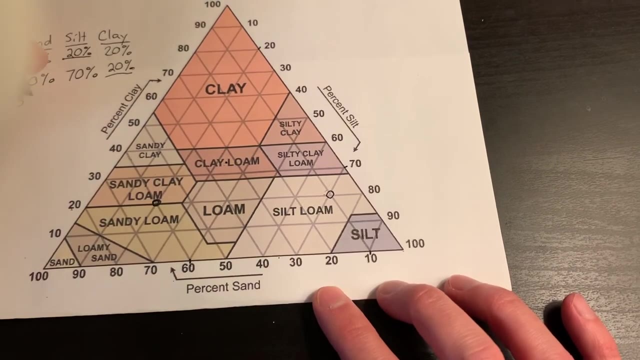 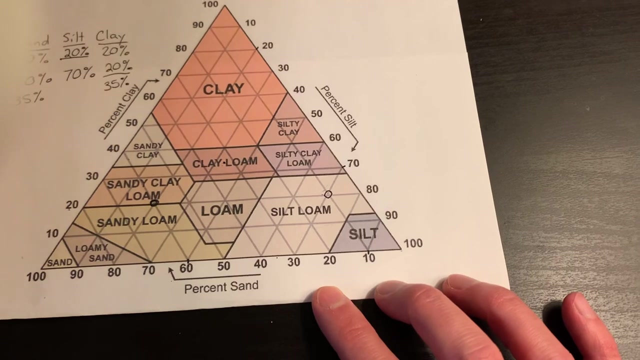 Right in the middle Doesn't have to be on the line, It can be in the middle. We take a look And we can say: clay loam, perfectly balanced clay loam would be about 35 percent sand And it would be about 35 percent clay. 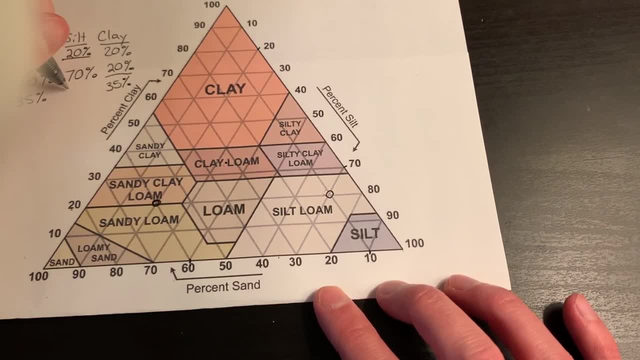 And obviously we know it's more like 33 and a third And we can say clay loam, Perfectly balanced clay loam would be about 35 percent sand And it would be about 35 percent clay. So there is our clay loam soil. 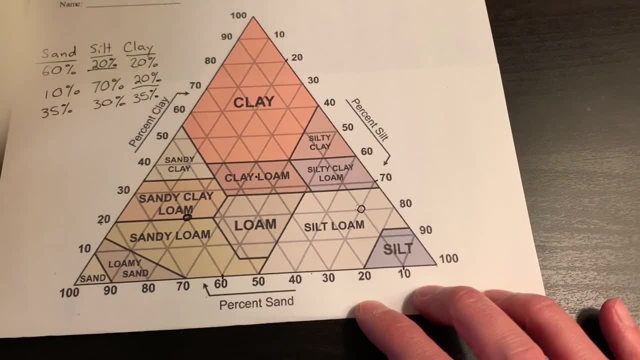 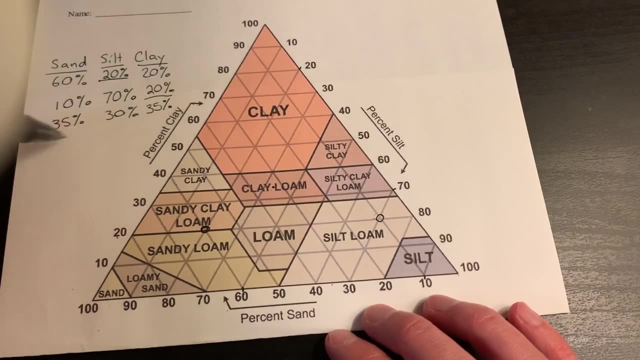 So this works in both directions And whatever your separate percentages are And whatever your separate percentages are, you use that to give you a classification of texture. You use that to give you a classification of texture.